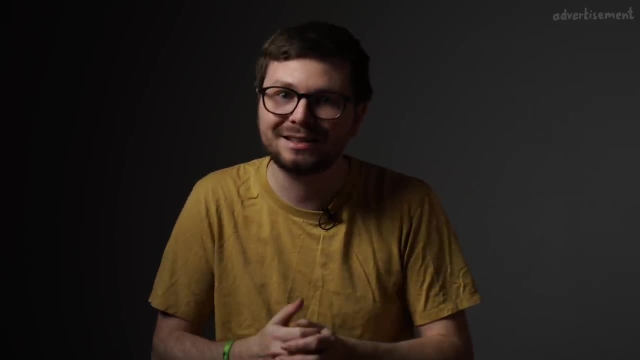 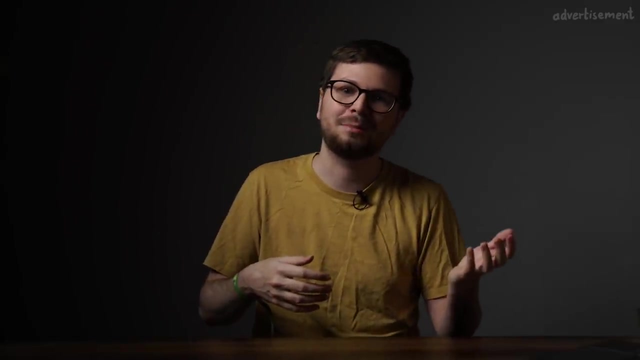 certain vulnerabilities and they always have a good reason why they decided they won't reward certain kind of reports. But it's a very fine line between what is a vulnerability and what is not a vulnerability. This is a difficult topic and you can argue about it a lot, So we made videos where 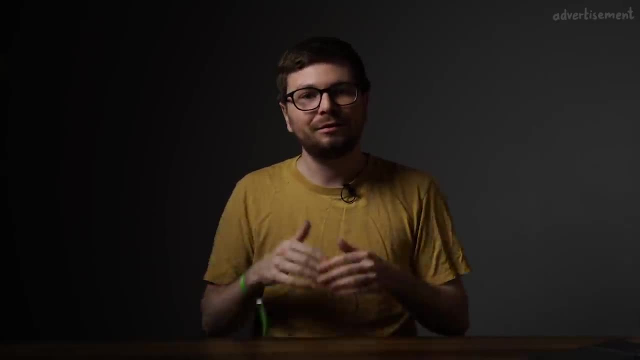 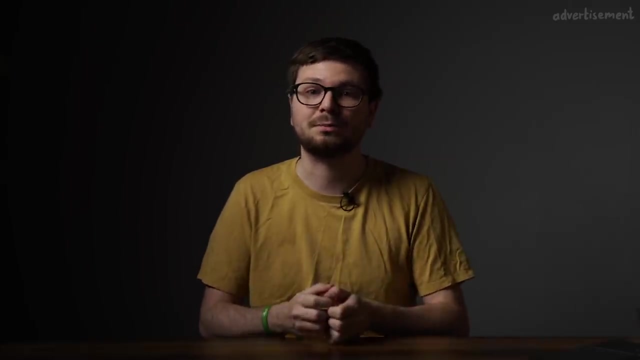 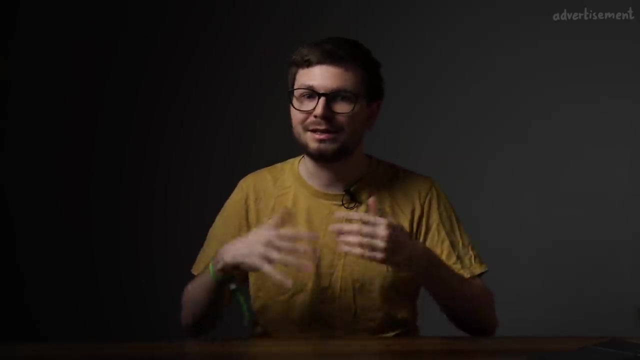 we tried to explain google's position And in the video I'm going to share today, I talk about various http security headers, Including cookieflash text and course misconfiguration, And I'm going to be a bit more critical about them. As I said, there is tons of content telling you about why they matter for security And, of course, 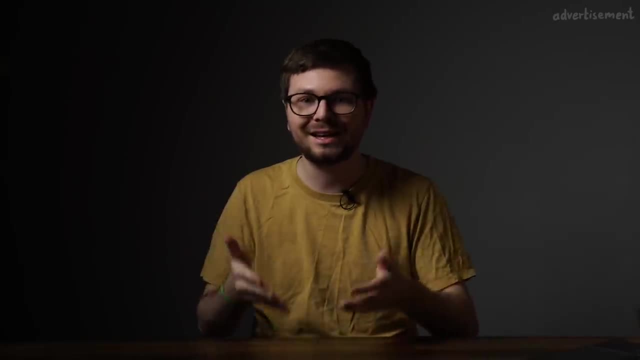 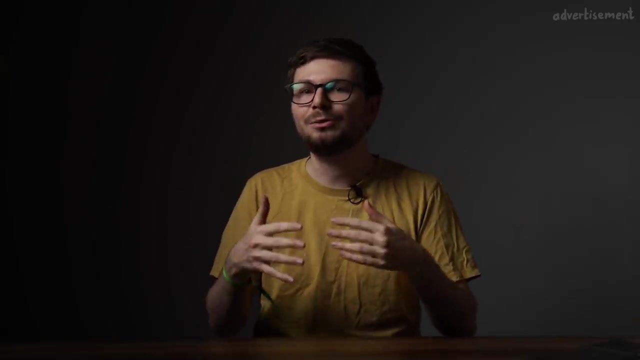 that material is not wrong- Of course they exist for good reason- But there is basically no content that tries to balance the sites a bit, And so in this video I try to be like: calm down, chill, the world is not gonna end if a site didn't use certain security headers. 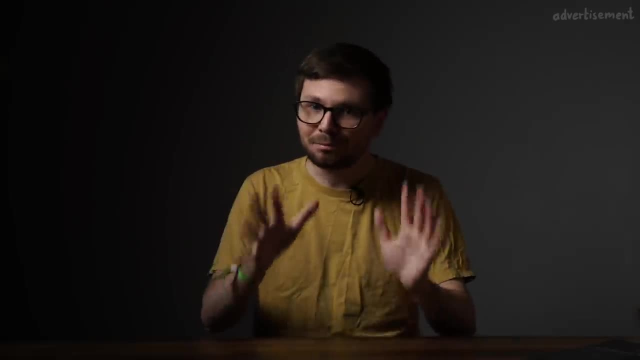 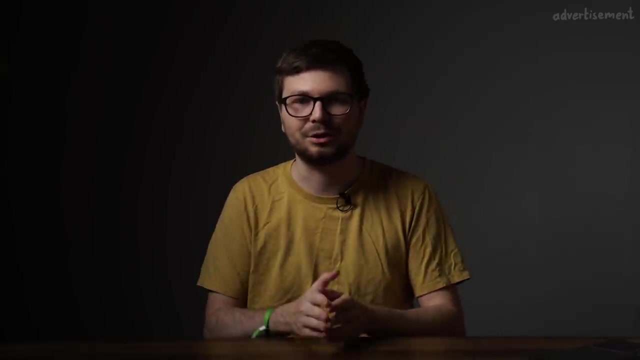 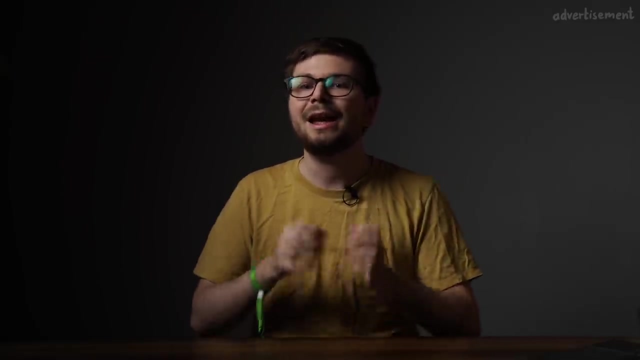 Also, I believe when you consider, at least for a moment, that maybe they are not so serious, it really helps to develop a deeper technical understanding about this topic. And even if you watch the video and in the end you say I still believe this should be reported, at least you have actually thought about the other side. 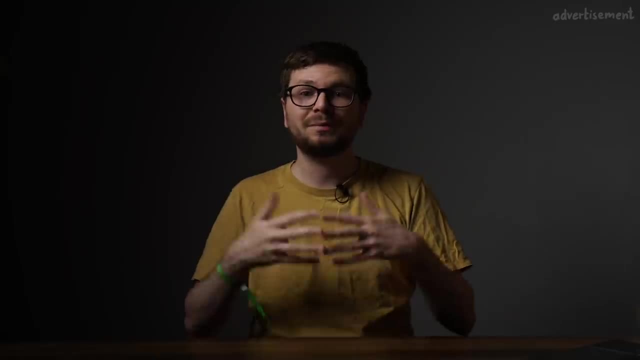 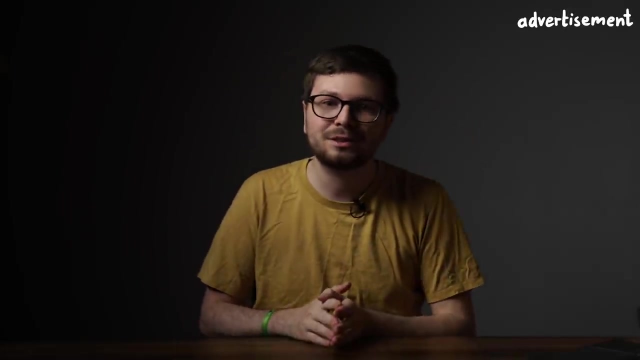 Anyway, two more things I wanted to mention about this video. First of all, this video was not meant to be an advertisement for google, but of course it kinda is. That's why I labeled it this way: Google paid for this video, but not to be shown on here. I know it sounds weird, but it's important. 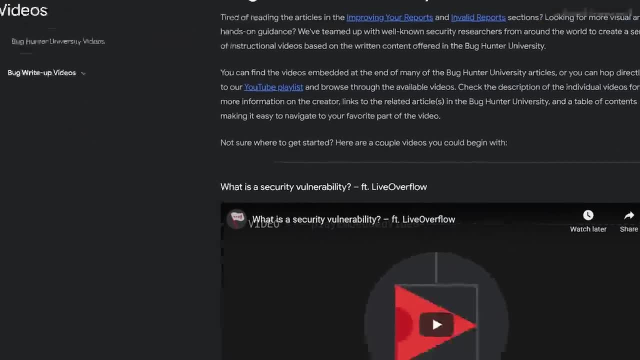 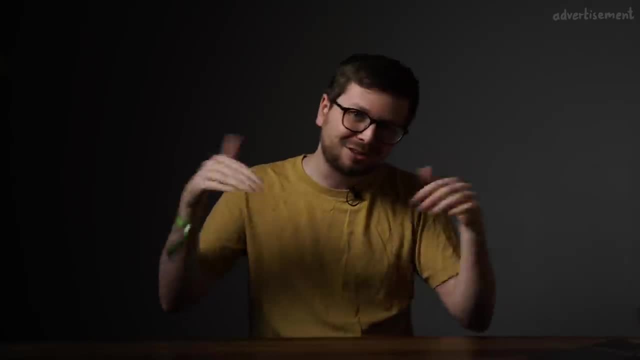 for me to mention this. This video was produced for google to be embedded on their site. It was not produced as an advertisement to be shown on this channel, But I thought my video is a very good educational video. I really like it myself and that's why I wanted to share it with my 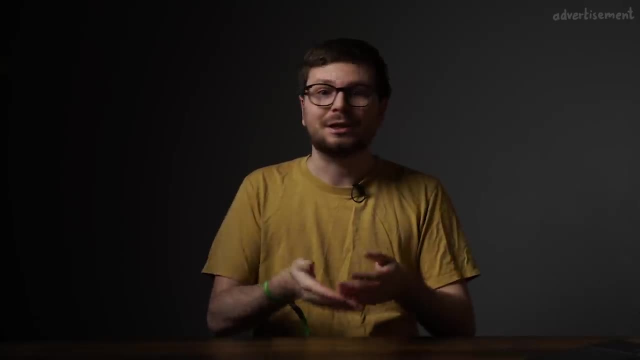 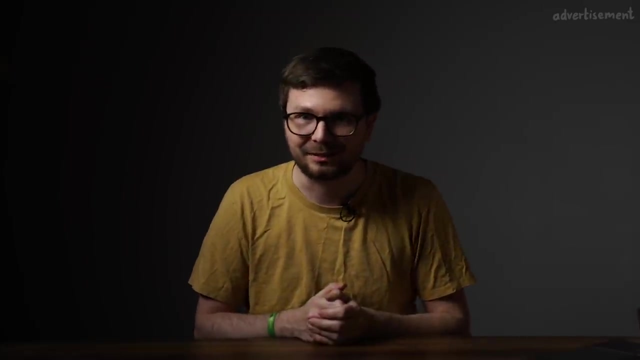 audience on here as well. So I'm very curious if any of your opinions about HTTP security headers are relevant to this video. so make sure to leave some angry comments at the end. And second, this video was made before I got my glasses. 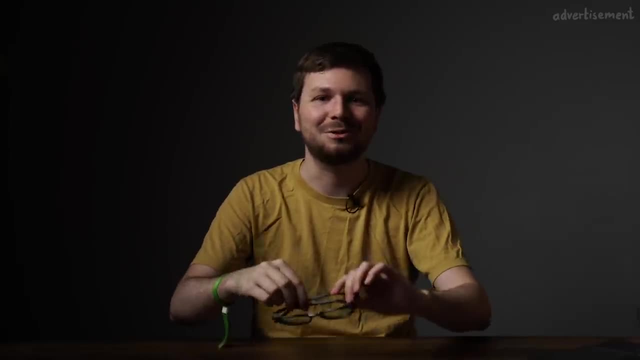 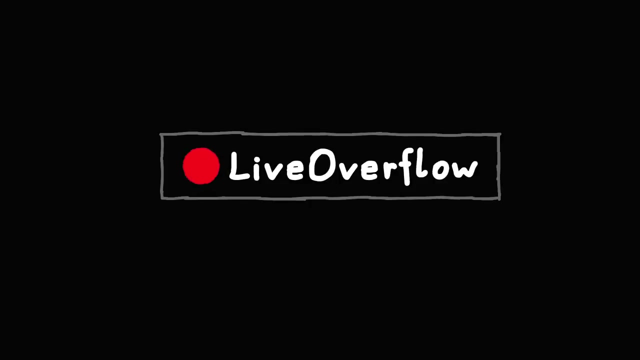 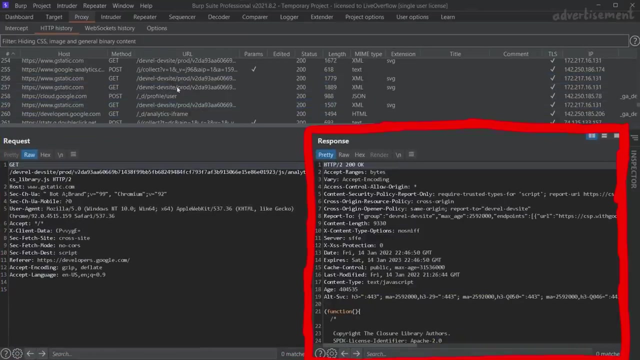 so I guess I take them off now to make the transition into the main video less awkward. When you are hunting for bugs, you probably look at all the HTTP requests and responses And they contain a lot of HTTP headers. The response headers are especially. 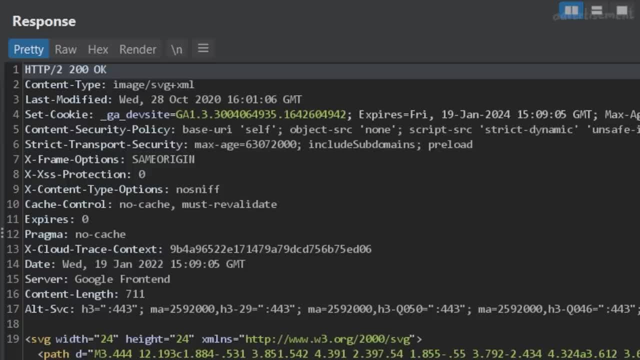 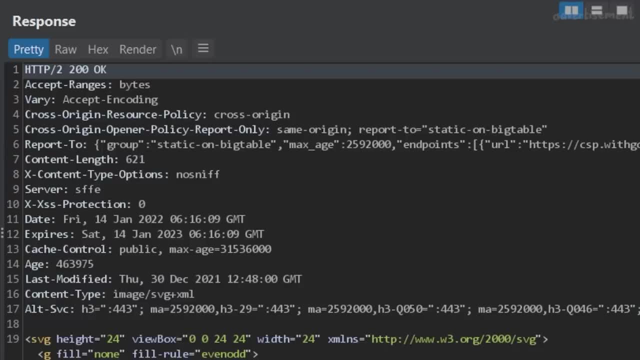 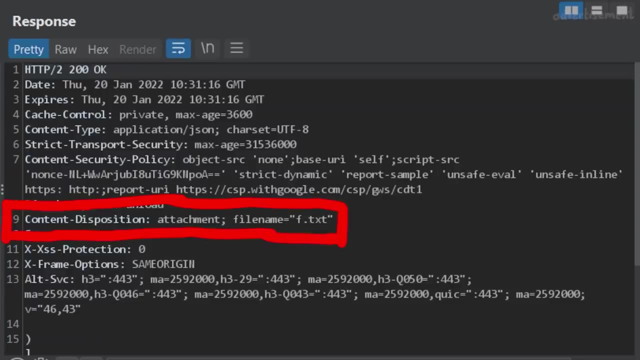 important as they can contain interesting information from the target. For example, it might tell you which web server is running. Other response headers are important for the functionality of a webpage, such as the content type, telling the browser how to interpret the response, or the content disposition header, which tells the browser if a returned response. 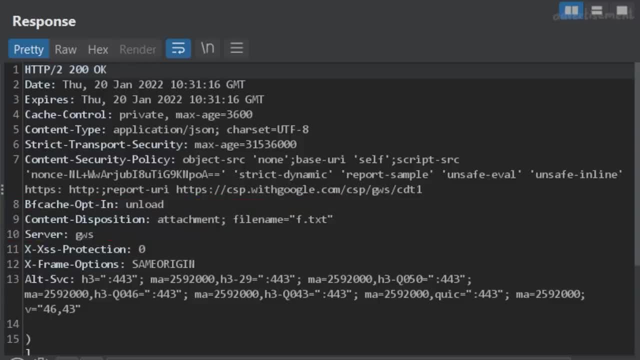 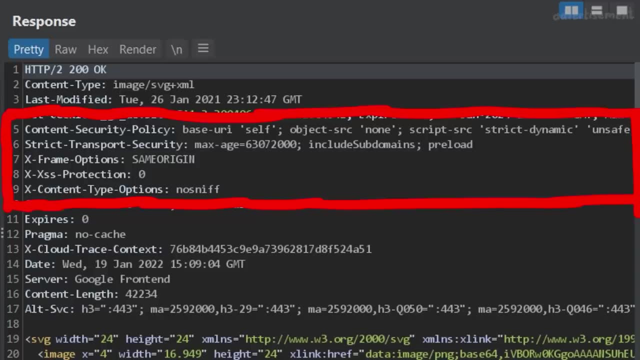 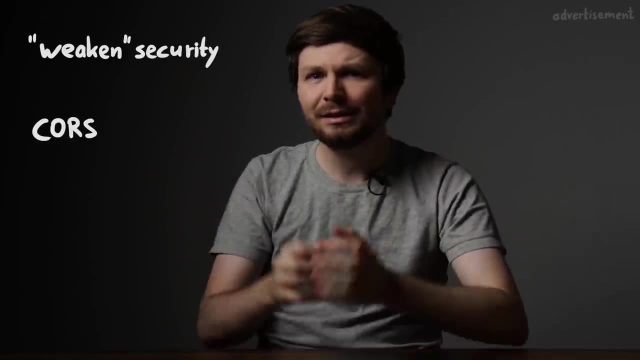 should be just shown or be downloaded as a file. But also some of these headers are so called HTTP security headers And they can be important for security. HTTP response headers can be placed in two categories: Headers that can weaken the security if they are added, And headers that strengthen security when they are added. 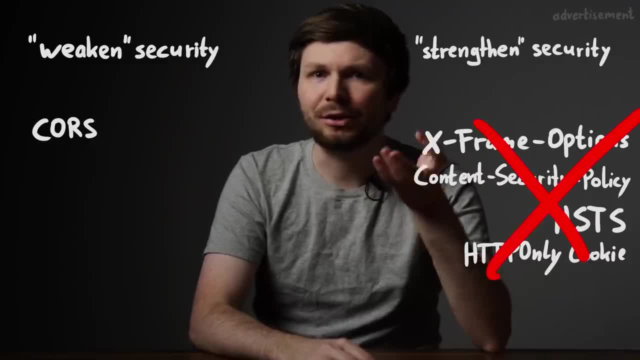 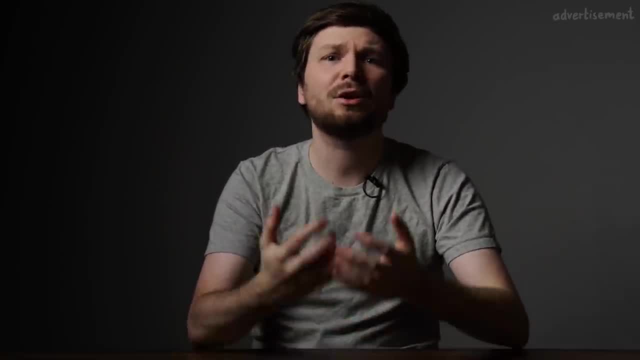 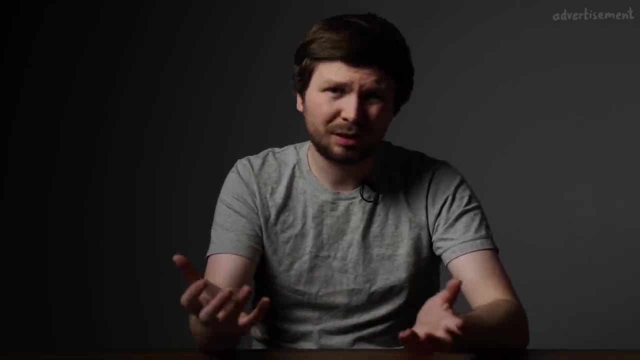 So the big question is now: if a site does not set certain security headers, is that a vulnerability? Online, you find many guides on best practices on what headers to set or not set. So if you identify such a header, could this be reported to a bug bounty program? 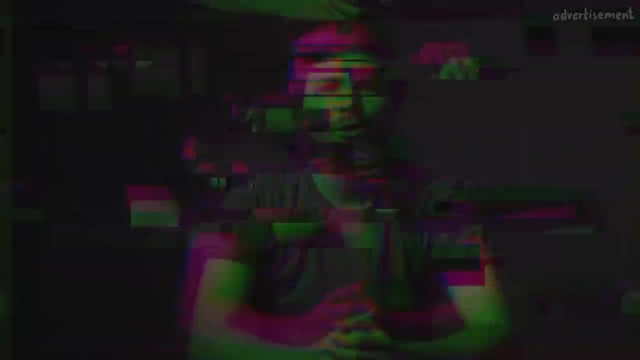 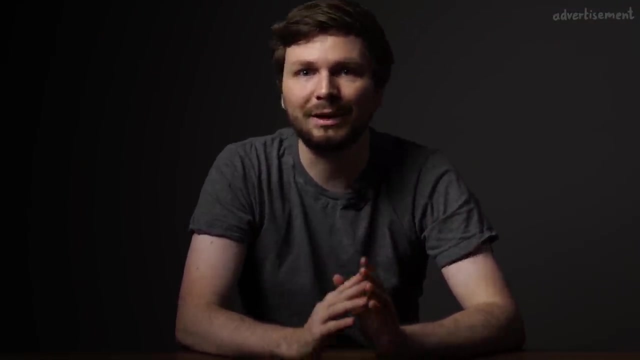 Let's learn more about HTTP response headers for bug bounty. To figure this out, we have to look at a few security headers in detail to understand what exactly they are doing, and only then we will be able to assess if it's a vulnerability when they are not set. Example 1. XFrame options. 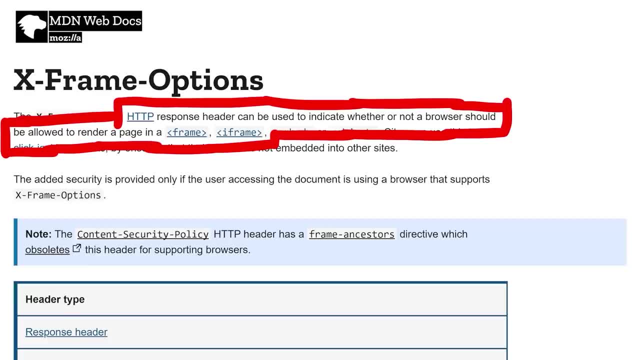 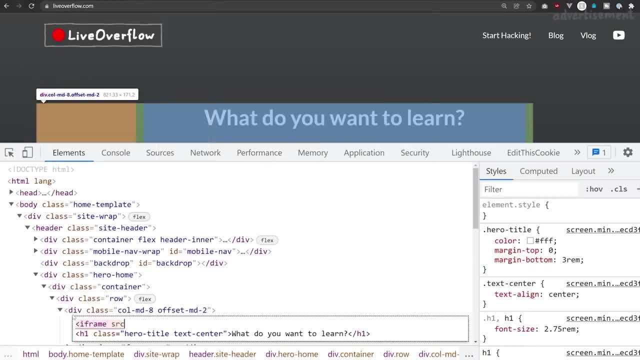 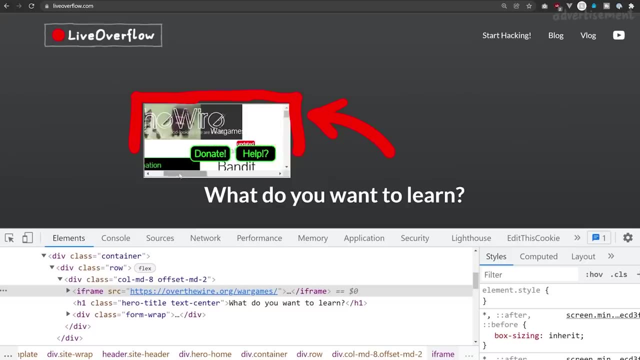 The XFrame options HTTP response header can be used to indicate whether or not a browser should be allowed to render the page in an iframe. With the iframe HTML tag, you can embed another website into your website, And this could allow an attacker to perform a so called click checking. 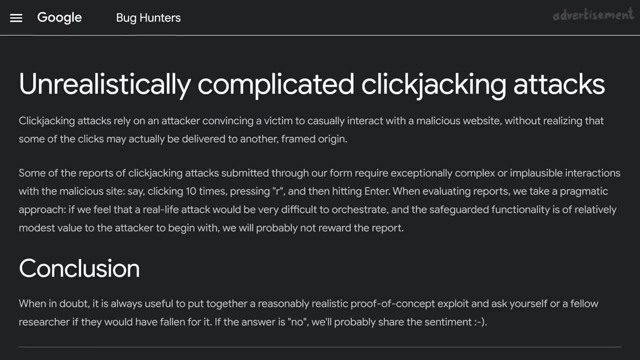 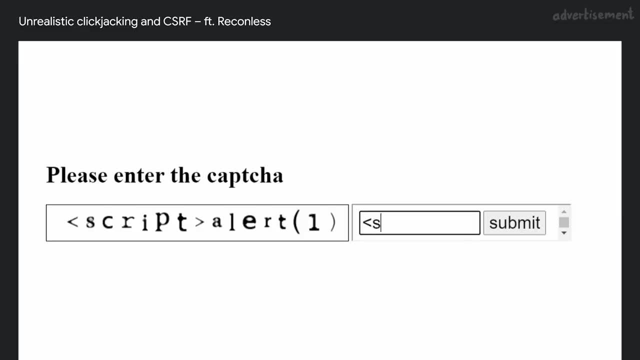 attack. If you don't know what click checking is, check out this article, which also has a great video from reconless explaining it. But they also explain why click checking is not a very serious vulnerability and why often it is not accepted for a bug bounty reward. 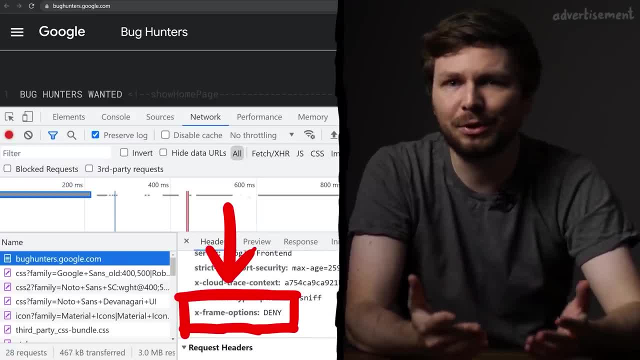 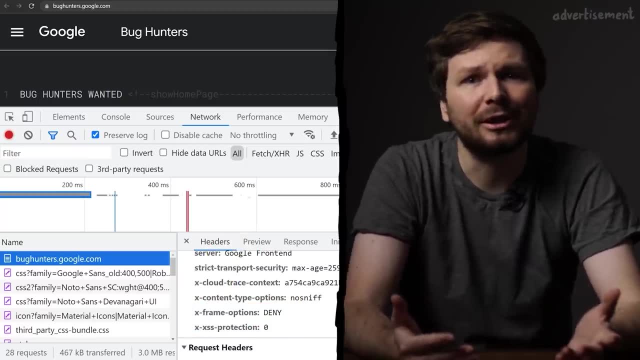 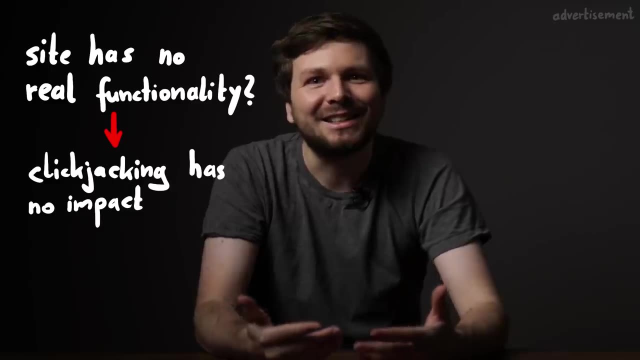 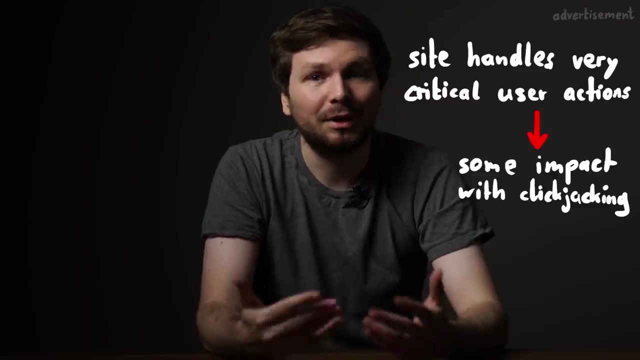 The thing is, yes, setting the XFrame options header in the response to same origin or deny would prevent such an attack, But that's not the only way you can prevent such an attack. Generally speaking, very critical functionality on a site, plus click checking, can be a vulnerability. 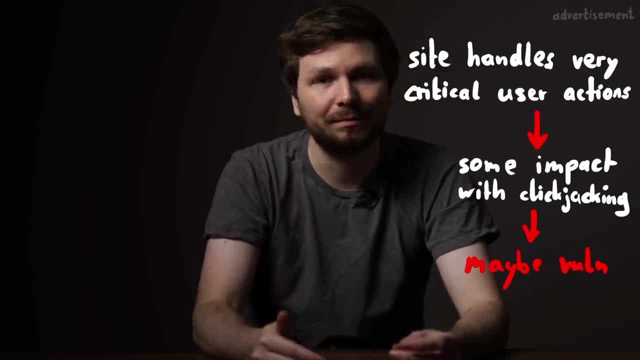 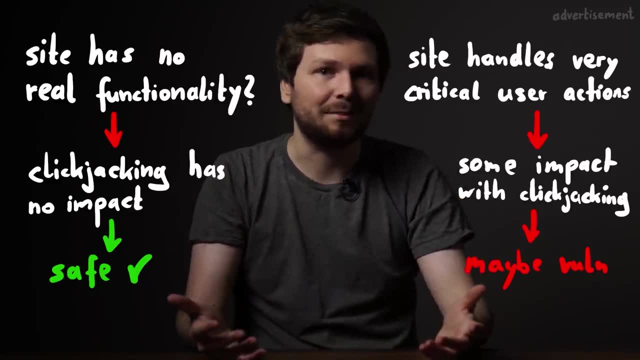 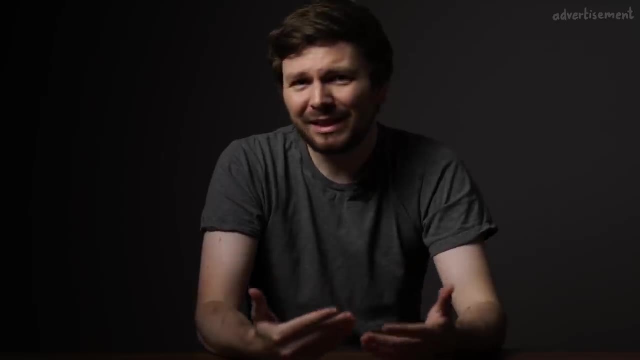 Then setting the XFrame options header makes sense. Boring and less critical actions available on a website plus click checking, doesn't matter that much. Setting the header in many cases doesn't hurt. it probably adds a bit of protection. but the missing header doesn't necessarily open you up to a text. You have to understand that. 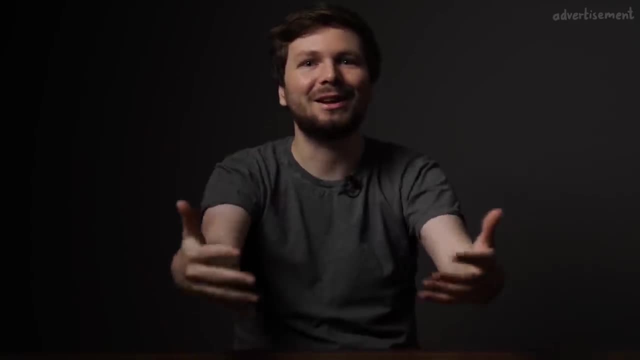 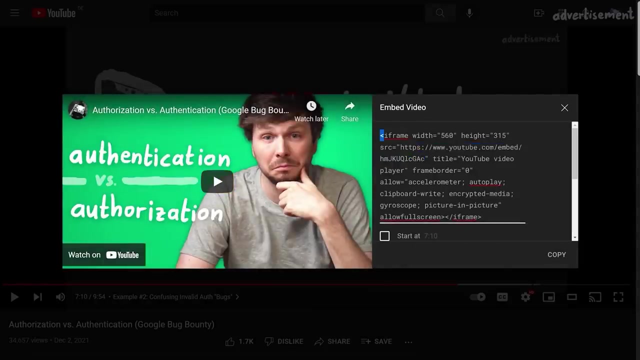 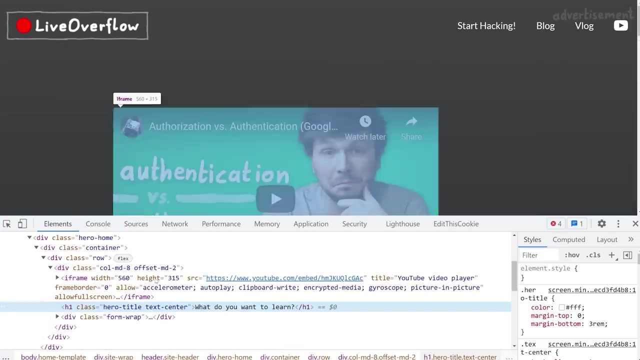 And then, of course, there are cases where the website wants to allow others to embed it. For example, on youtube, when you click on share, you copy an html snippet for embedding the video and it has an iframe tag. So youtube wants you to be able to embed the content. It's a feature. 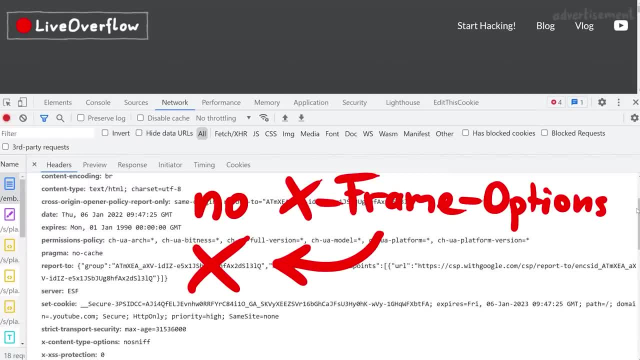 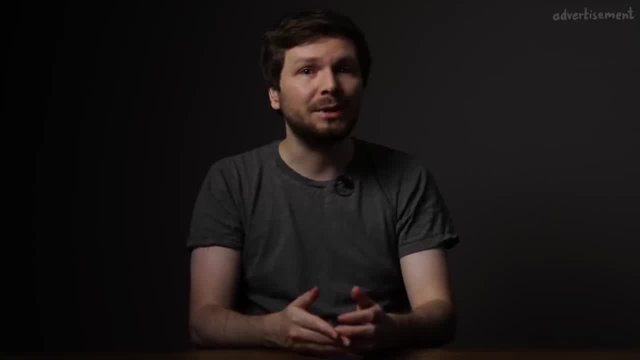 And, of course, in that case, they don't want you to be able to embed the content. They want you to be able to embed the content. So you can see, it depends on the context of the website if it's important for this header to be set or not, Which means you shouldn't blindly follow. 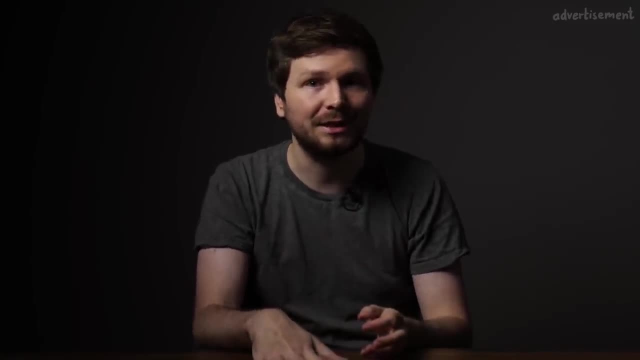 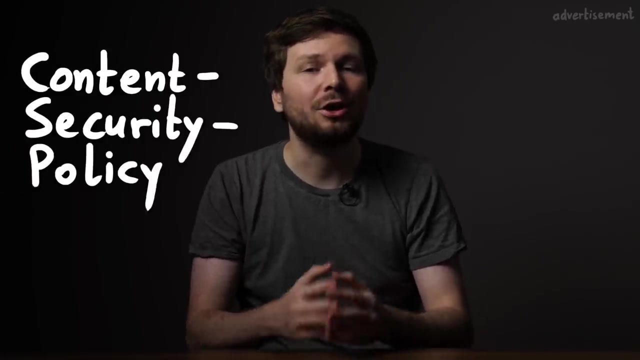 best practice guides or scanners that tell you that the header is missing. You need to understand if there is actual impact- Example 2.. Another important security header is the content security policy, CSP. And CSP is awesome because theoretically it can protect your website pretty. 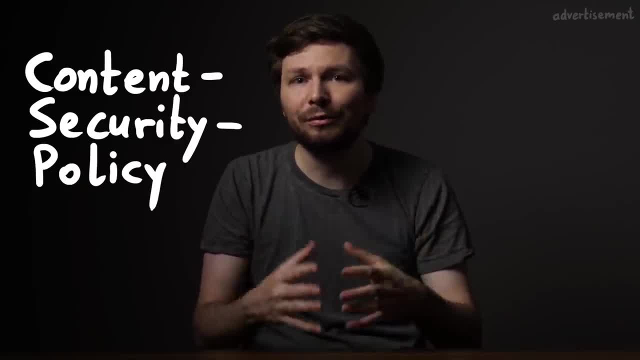 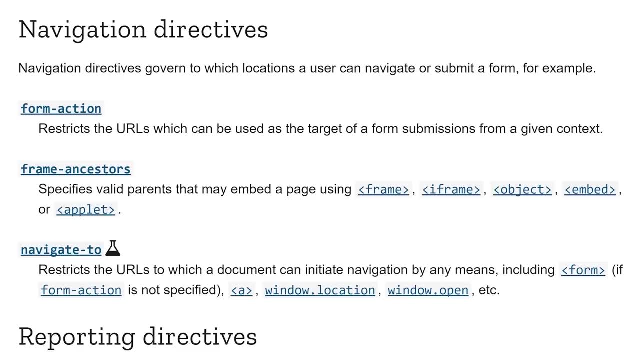 much from any cross-site scripting attack And it even has more features beyond XSS. With CSP you can also set the frame ancestors to none, which kinda acts like setting the XFrame options header. So if CSP could block XSS, wouldn't it be a very important header to set? 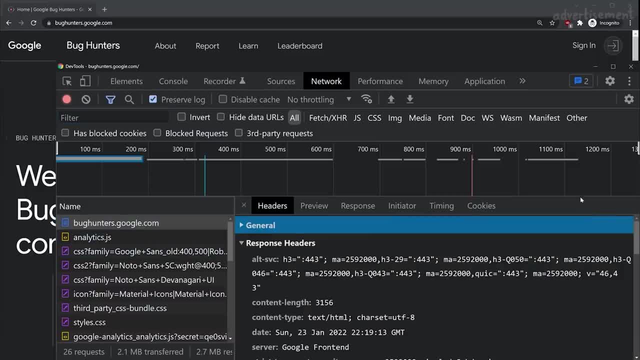 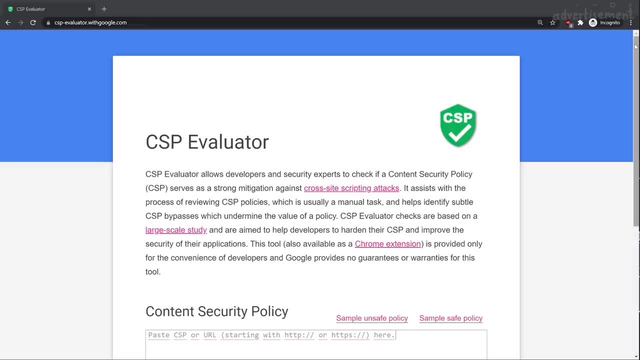 Let's do an example and let's go into the google bughunter site and have a look at their CSP. Huh, There is no CSP. There is this awesome tool from google engineers called CSP evaluator, and it can help you to assess a gist of what's going on in your website. 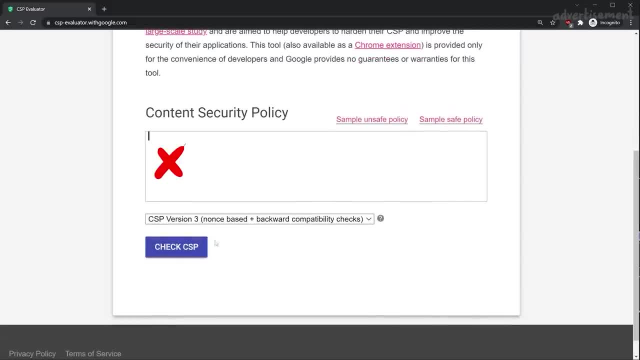 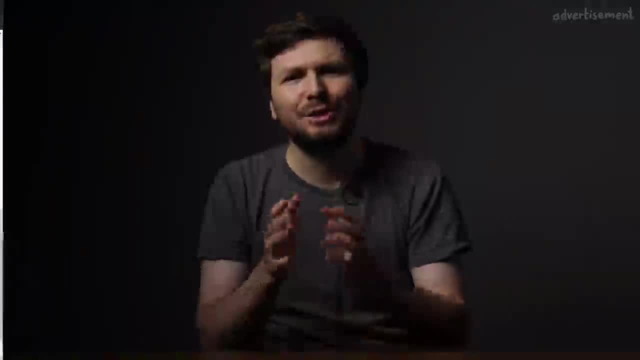 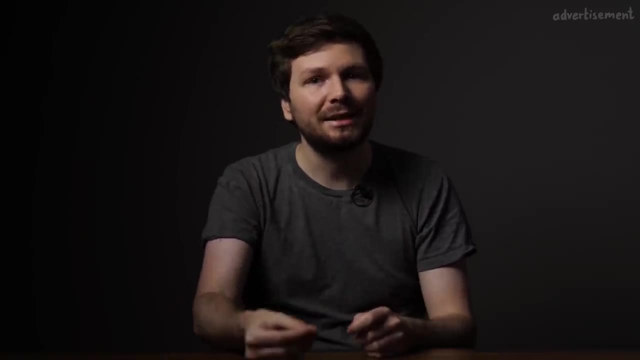 In this case, there is literally no policy. So let's submit an empty text and the tool reports a high severity, finding Script source missing. So is this a vulnerability in itself? Well, as I said, CSP can protect websites from XSS attacks or other kinds of attacks, But because CSP just protects, it doesn't. 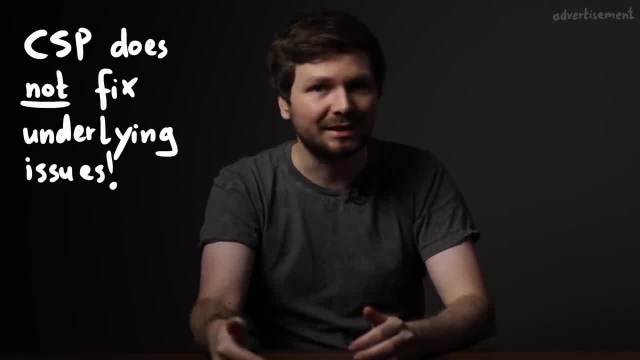 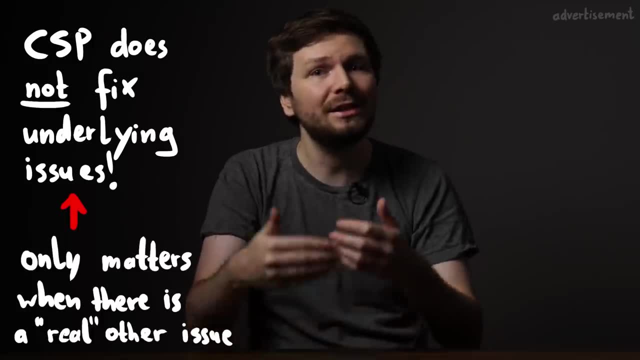 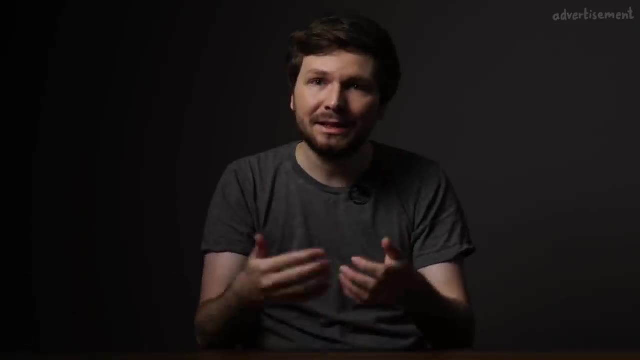 make it a fix for an issue. If there is an XSS, CSP doesn't fix it. It could just block exploitation. It's a defense in depth strategy. So setting script source CSP only matters in the context of an XSS issue existing in the first place, And that means missing CSP header in. 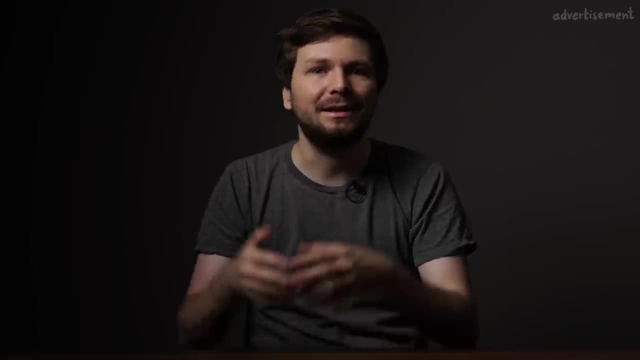 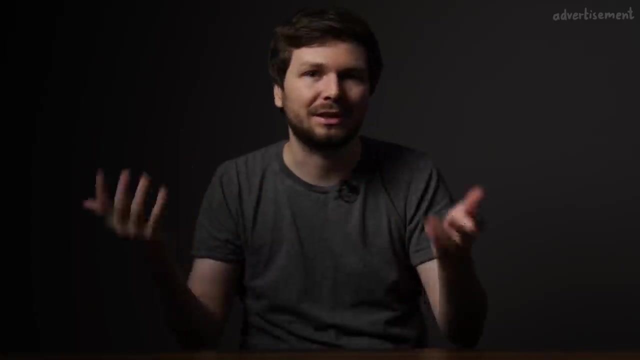 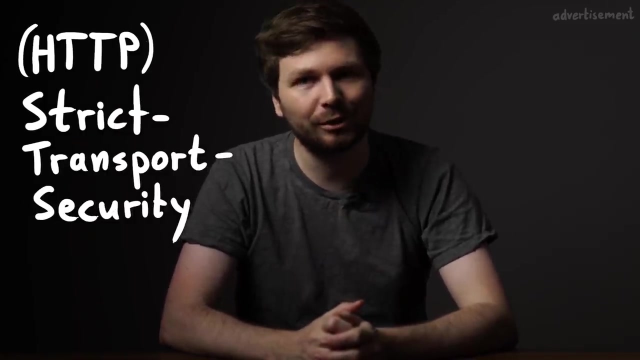 itself is not really a vulnerability. Again, it depends on how critical the website is if this protection is really important or doesn't matter. Example 3.. Let's have a look at another header: HSTS, HTTP, Strict Transport Security. This really sounds like an important header to set, But what exactly does it do? 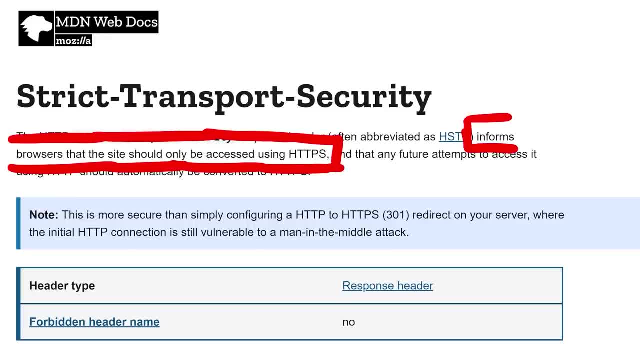 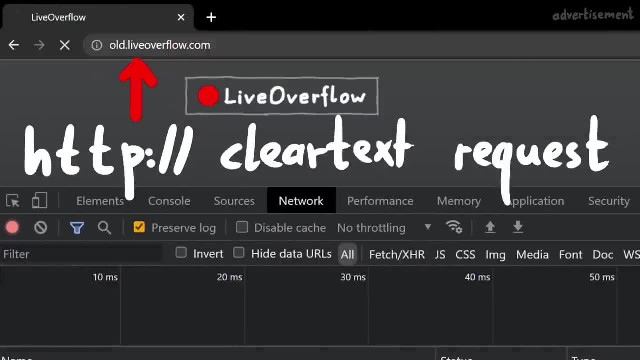 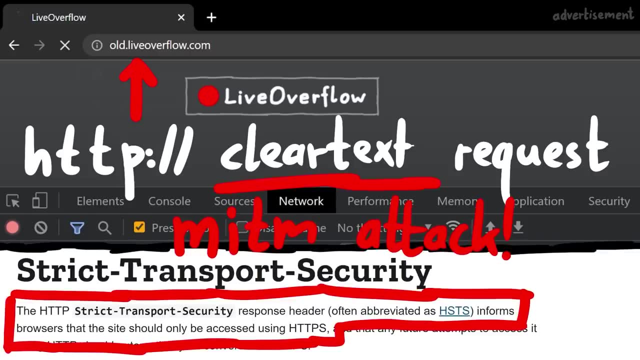 It lets websites tell browsers that it should only be accessed using HTTPS instead of using HTTP, For example, the visitor types wwwfoocom or even just foocom. This creates an opportunity for a man-in-the-middle attack. The http strict transport security header informs the browser that it should 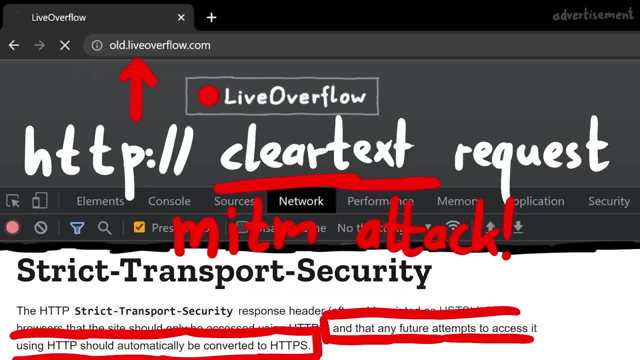 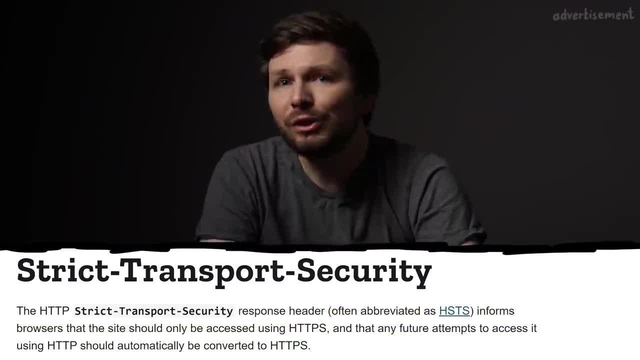 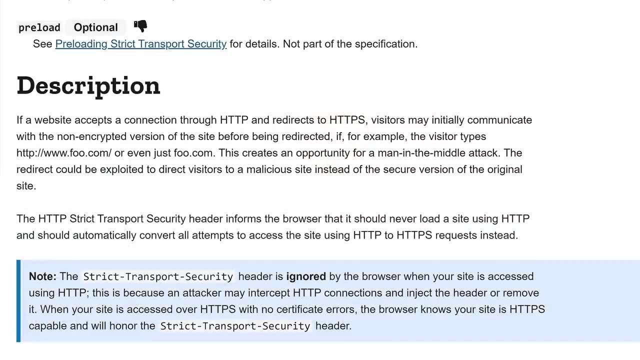 never load a site using http and should automatically convert all attempts to access the site using http to http as requests instead. This sounds very useful, But then why is it considered an invalid report if a site from google is missing it? Well, right below there is also this note: The strict transport security header is ignored by 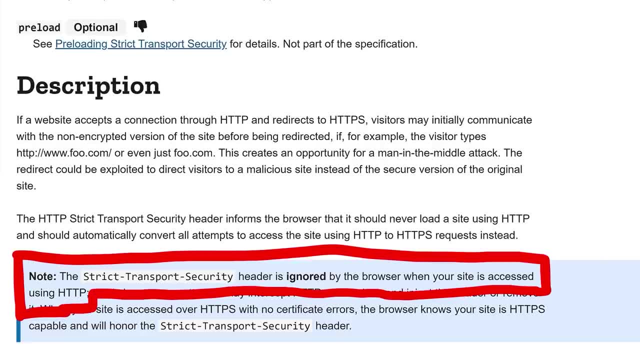 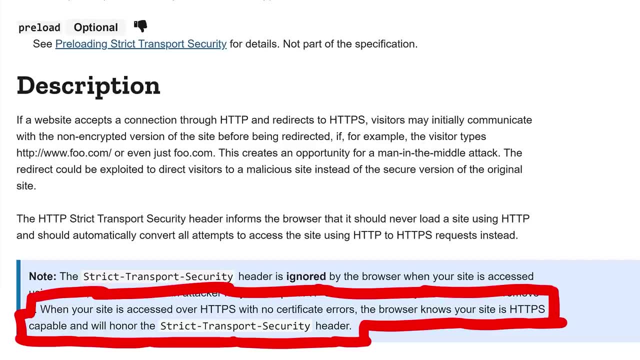 the browser when your site is accessed using http. This is because an attacker may intercept http connections and eject the header or remove it Only when your site is accessed over http. Yes, with no certificate errors, the browser knows your site is HTTPS capable and will. 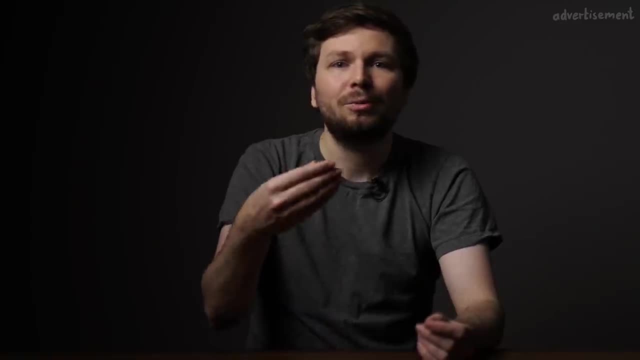 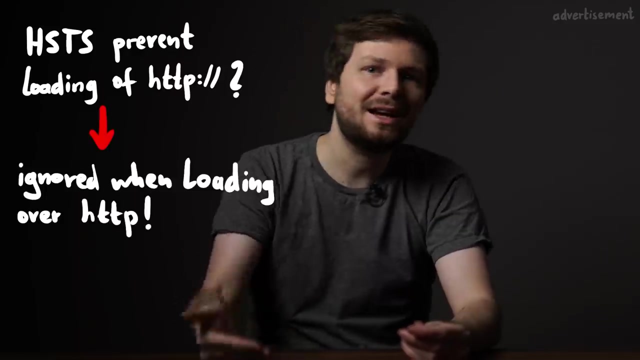 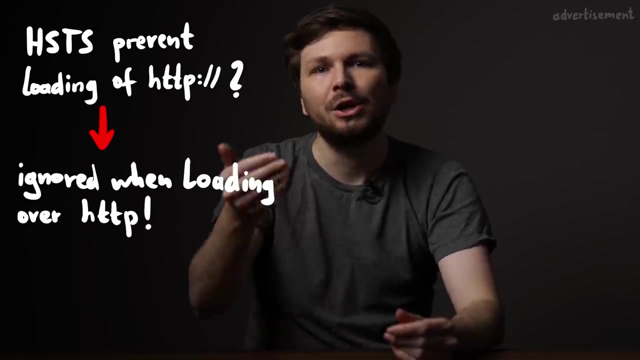 honor the strict transport security header. So we already have this weird situation where the header is supposed to prevent users from loading the site with HTTP, But if the site hasn't been loaded yet, the browser doesn't know about it and only honors it once the site was loaded securely once. Which, of course, is better than nothing. but modern browsers do the same anyway. For example, when I visit liveoverflowcom with an HTTP URL, you can see that it tries to go to the HTTP version, but it was redirected to HTTPS. Now let me try to go to the HTTP version again. 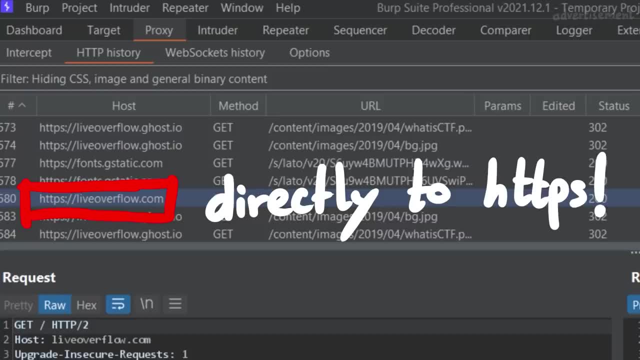 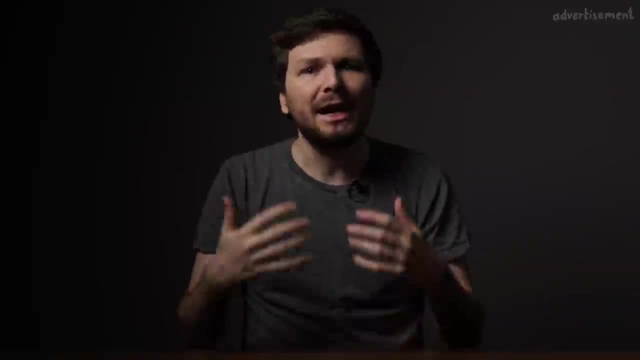 There is no HTTP request going on, We directly go to the HTTPS version. All of that without an HSTS header. So, as you can see, HSTS is not a silver bullet protection and browsers kinda mitigate it anyway, But it's still generally reasonable. 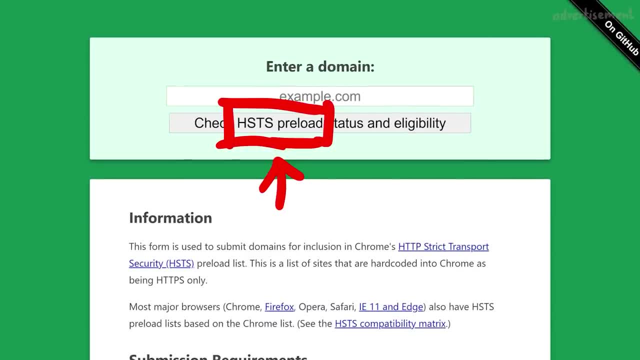 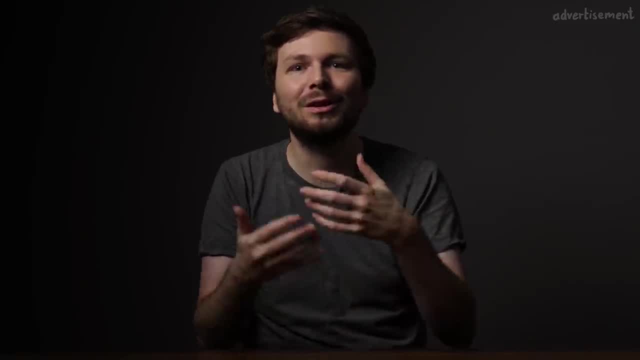 So let's go to the HTTP version. It's recommended, and especially together with the HSTS preload list, by the way, a project by google. it's good, But you also see that it's a very known and popular header. Google knows about it. 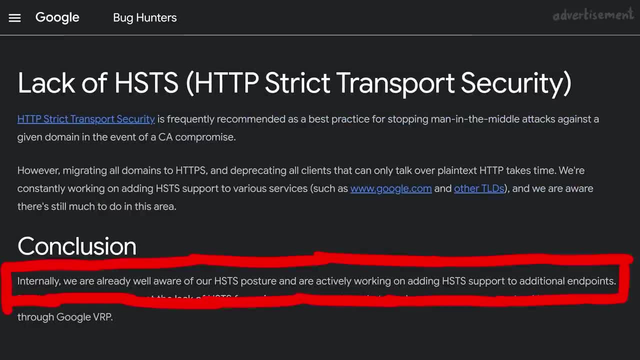 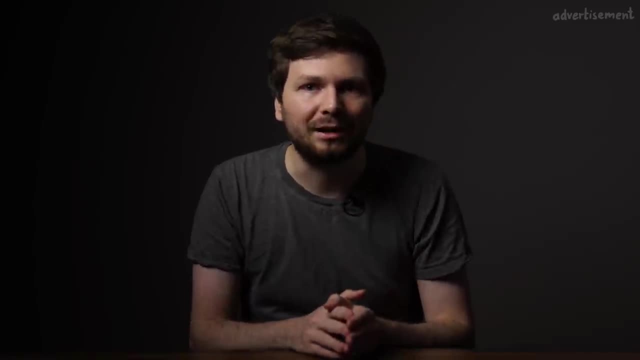 Which you can also see here in the article. Internally, we are already well aware of our HSTS posture and are actively working on adding HSTS support to additional endpoints, So it's a known issue to them. Next example: Coarse. Now we just talked about headers. 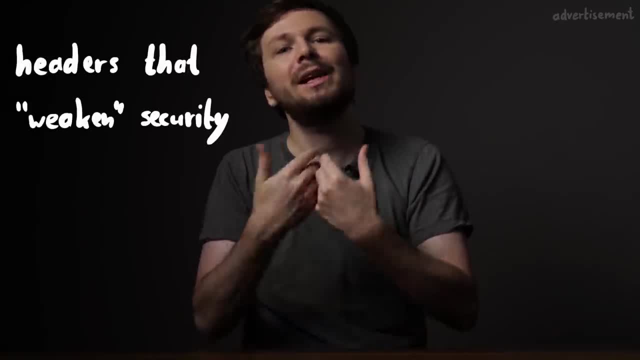 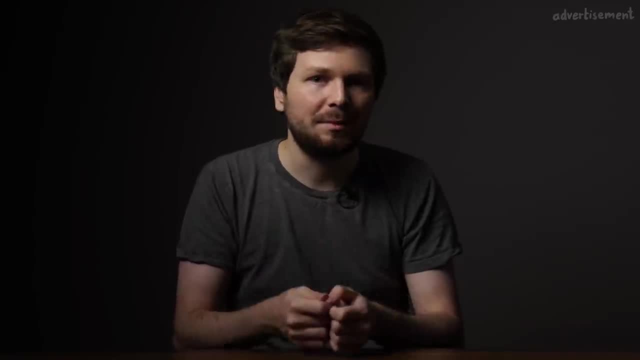 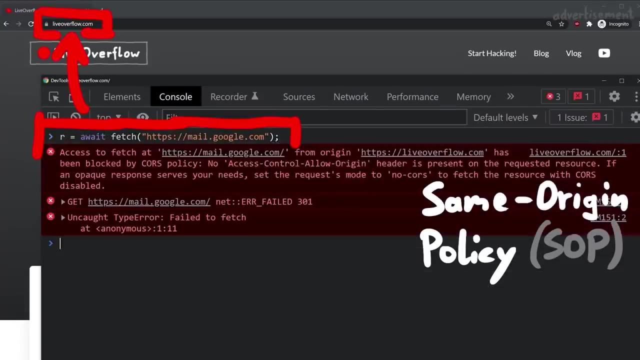 They add security to a site, But there are also headers that could WEAKEN the security of a site, And a very typical report is coarse misconfiguration. Generally, websites are protected by the same origin policy. This means javascript code on, for example, liveoverloadcom can not send HTTP requests. 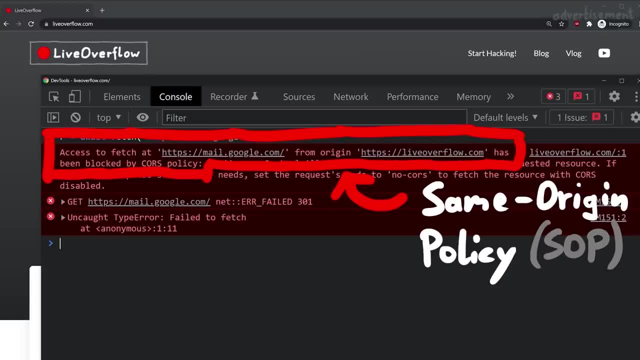 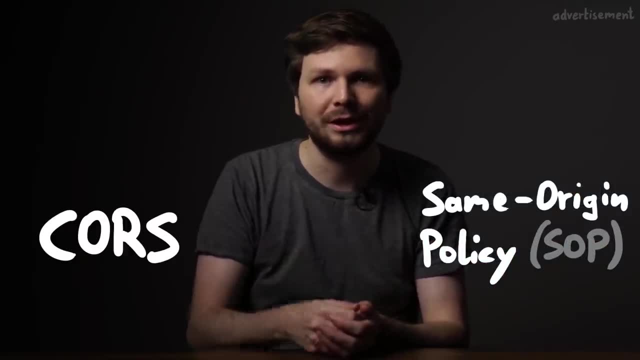 to gmail and leak your emails. The browser says no, I won't allow liveoverloadcom to access your gmail, But a webserver can use coarse headers- Crossoriginregistercom Source sharing- To actually allow another website to send requests to itself. 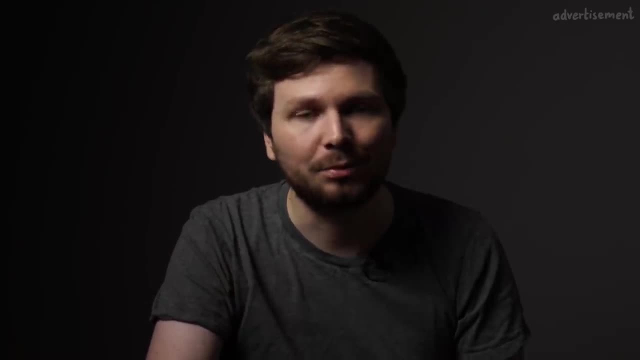 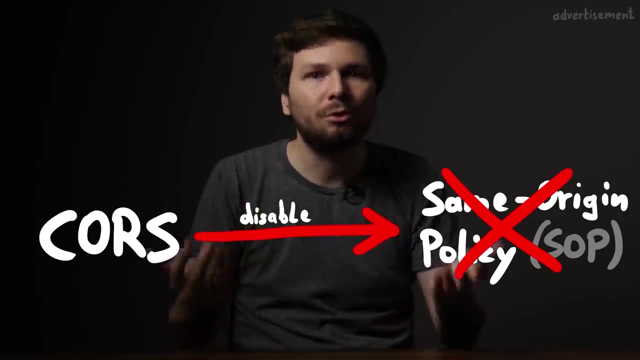 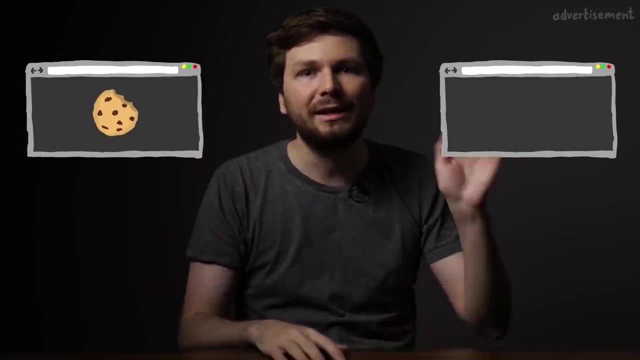 And at first sight this seems to weaken the same origin policy, Which it does. So why would anybody do that? Is there any negative security impact? It of course depends. Let's imagine two websites. One website uses cookie authentication. There is a session cookie. 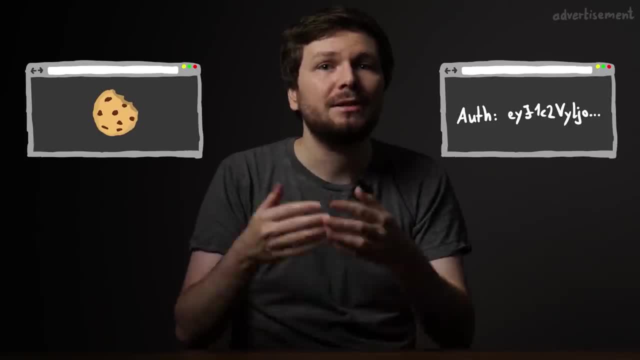 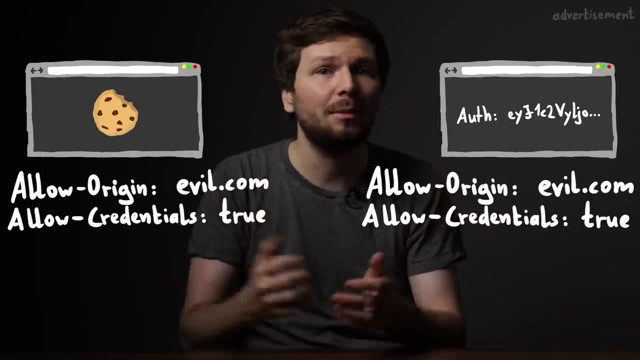 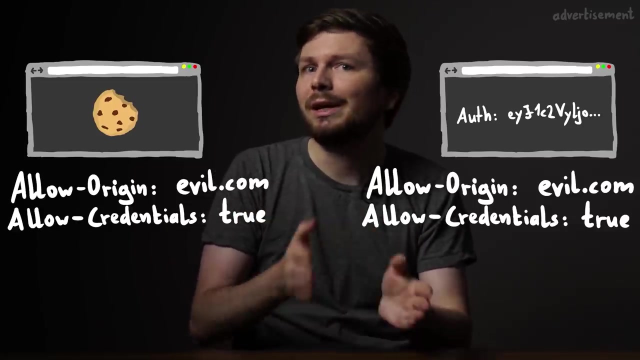 And the other website has token authentication. For each request, the code on the site adds an authentication header with a token. Both websites have very permissive, coarse settings allowing arbitrary origins to make requests And even allow setting credentials. Is this a security issue in both cases? 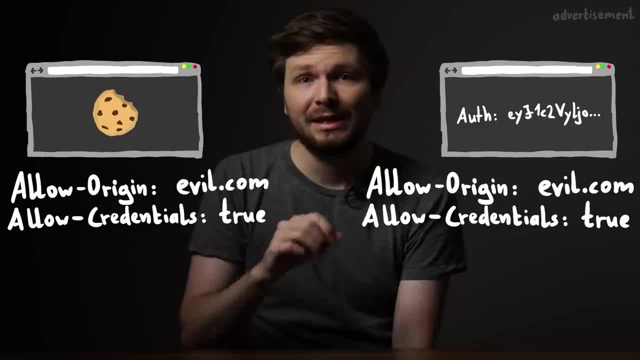 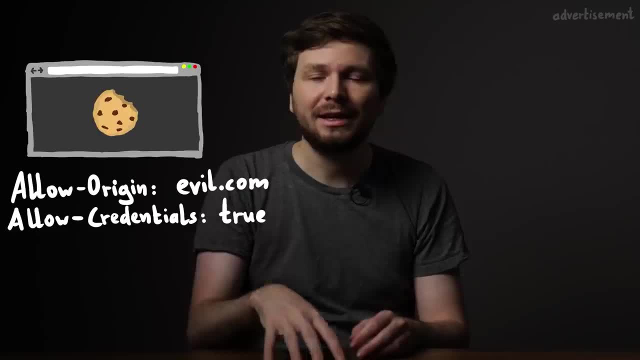 Only for one of them. this coarse setting is actually an issue. Setting access control allow credentials tells the browser that it can add the session cookie to the request, So in this case the request would be authenticated as the current user and the security impact of this. As you can see, This is really bad and definitely a security issue. But for the other website with token authentication, there is no session cookie. The browser doesn't set the authorization header for you. This request would not be authenticated as the user. thus there is no CSRF like attack. 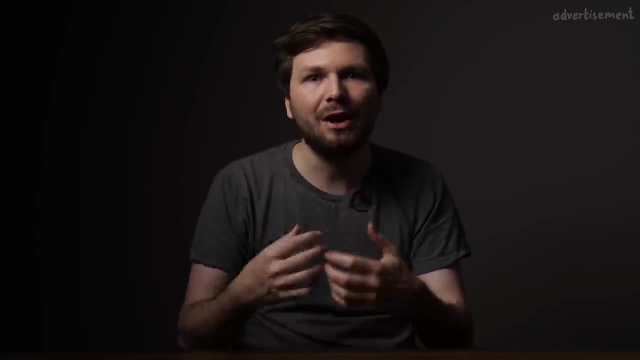 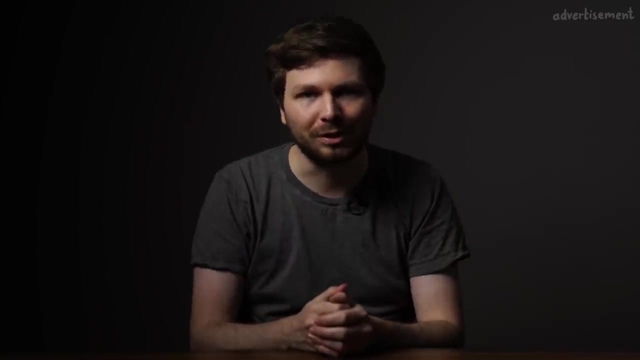 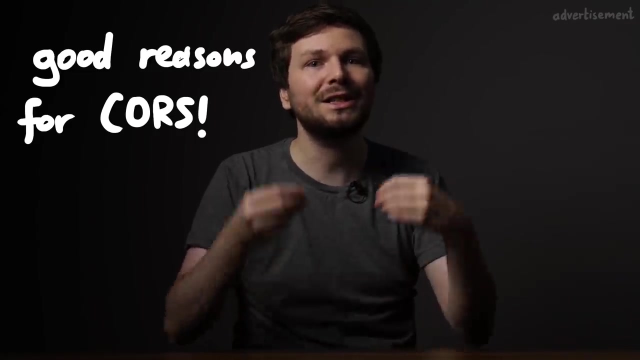 possible, As you can see Context matters and you have to understand if there really is any impact And you cannot blindly report an open, misconfigured course. So keep in mind that course exists for good reasons. Many websites from google allow course requests because it's meant as an open API, that is. 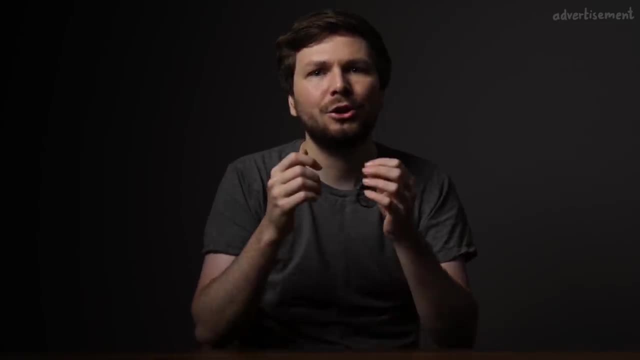 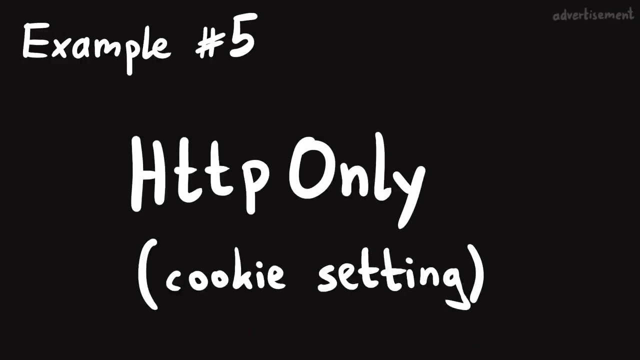 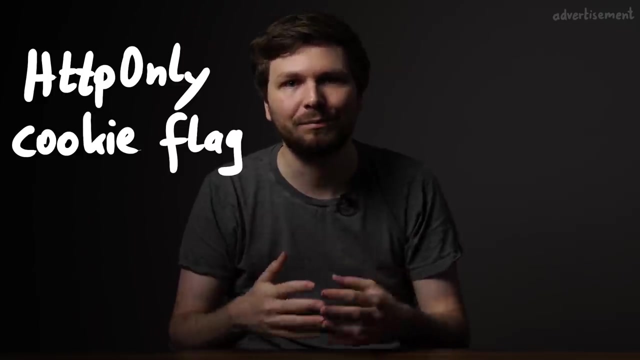 intended to be accessed from other origins. So you always need to be sure that there is really security impact. And the last example: HTTP only. Before we have a summary of this video, I briefly wanted to mention the http only cookie flag as well. 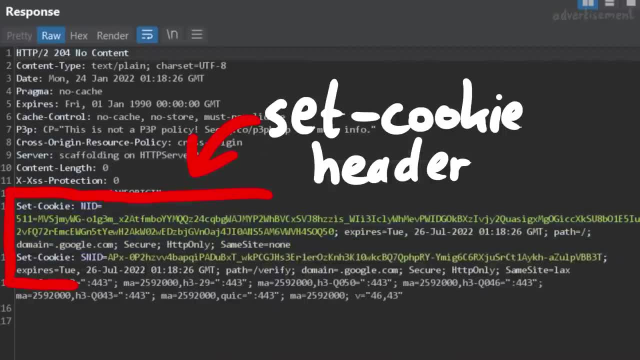 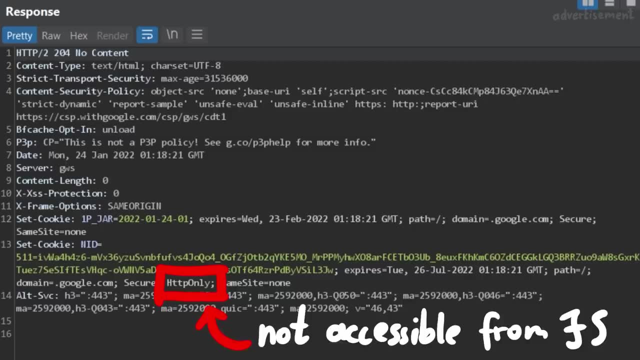 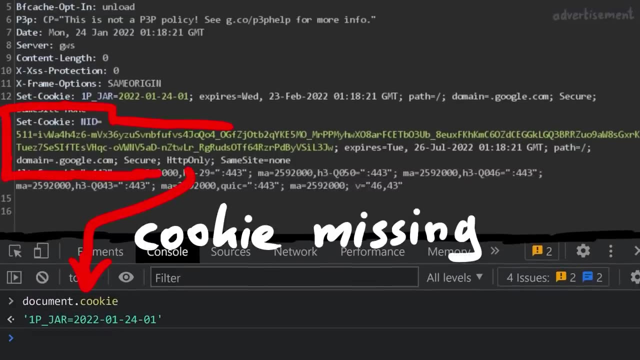 Cookies are technically part of the headers, So it fits into this video And the setting causes cookies to only be transmitted in http requests and cannot be read from javascript. It often is considered a defense against XSS attacks stealing cookies, But it's rather ineffective. 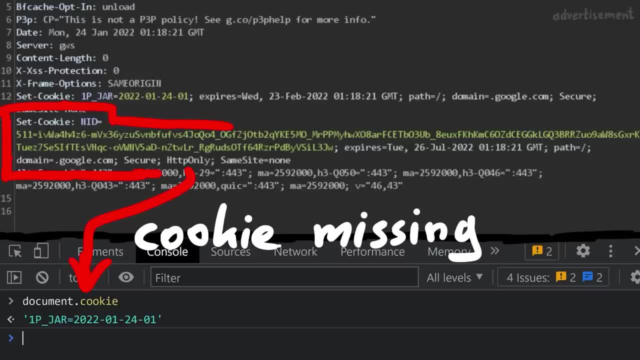 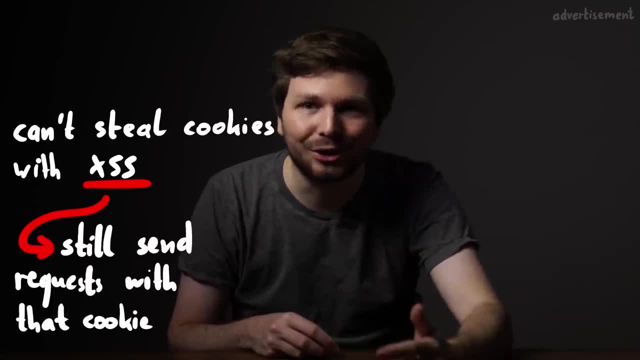 Yes, the cookie cannot be stolen, So you, as the attacker, cannot perform requests, But it's rather ineffective. Yes, the cookie cannot be stolen, So you, as the attacker, cannot perform requests as a user directly. But when you have XSS, the XSS can just send the requests you want for you. 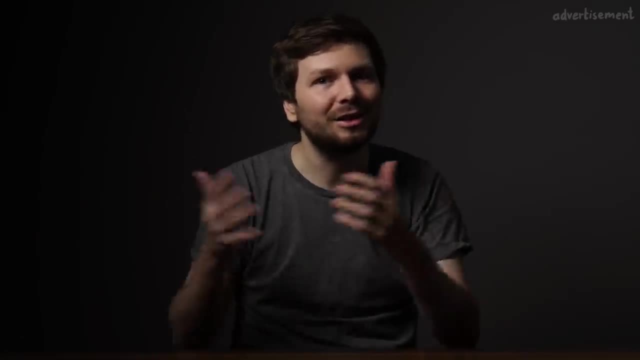 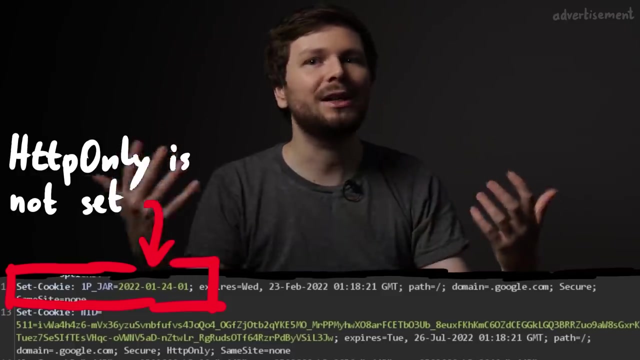 And those requests will be authenticated. So it's really not that big of a deal. And, on top of that, not every cookie is really used for authentication. Cookies are a great way to store a bit of information about a user and the app. They don't really have any security relevance. So if they are missing the http only flag or even the secure flag, It doesn't matter. So, as always, you have to really understand what a cookie is for and if there is really any impact. 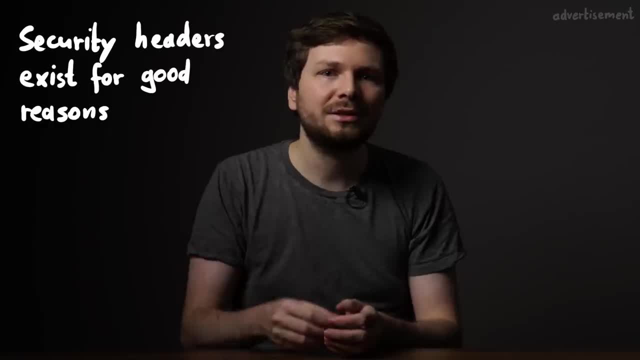 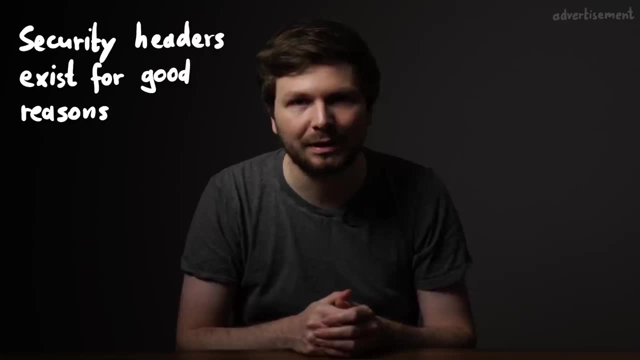 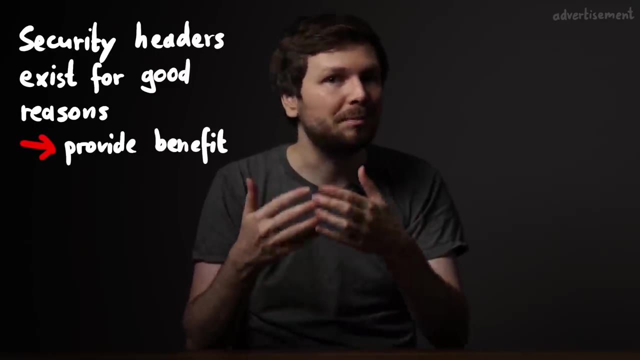 So let's summarize what we learned. There is a reason these security headers exist. They do really good things and can protect an application from exploiting other vulnerabilities, But them missing doesn't necessarily create a vulnerability. Most websites probably could benefit from setting some of them. 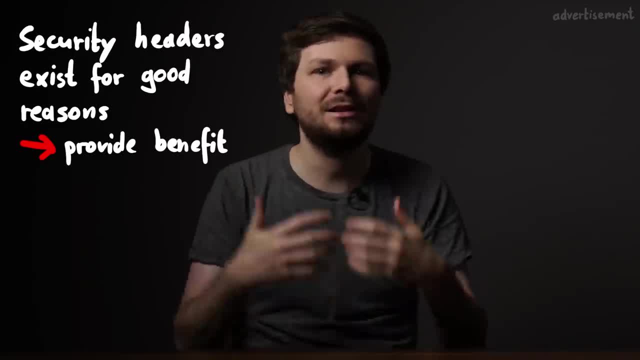 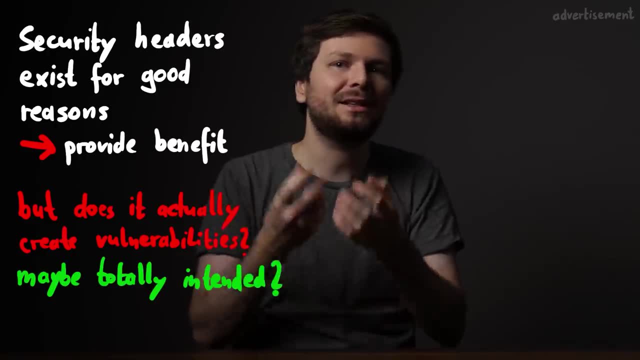 But most websites probably could benefit from setting some of them. But it depends a lot on the context. You have to understand the functionality of a website to judge if there is a significant risk And if it even makes sense to set them, Because maybe there is an intended feature why they don't want it. 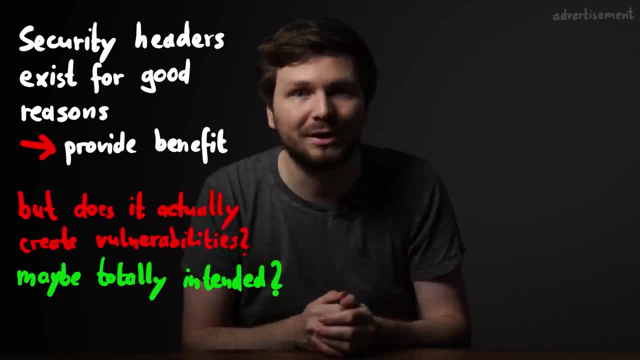 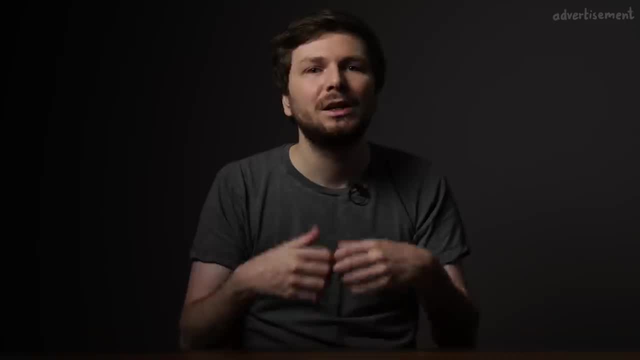 For example, youtube embedded videos that deliberately don't want to set the xframe options. You cannot blindly copy and paste the result of a scanner reporting that headers are missing. So make sure to read and understand what certain headers do, and make sure you understand if